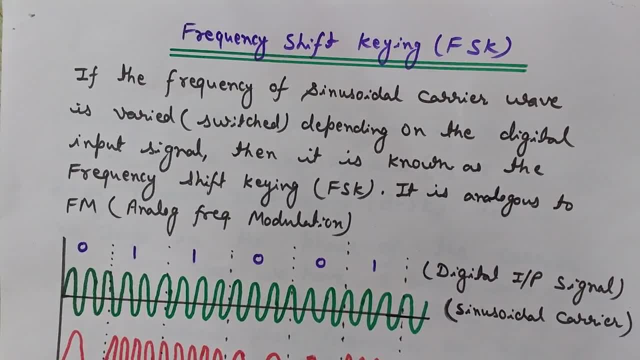 signal, The modulating signal here, is digital in nature, So the input signal is digital. You can see, here it is in the form of zeros and ones. Okay, So if we talk about binary FSK, then we have only two symbols, That is zero and one. First symbol is zero and another is one. That's why it is known. 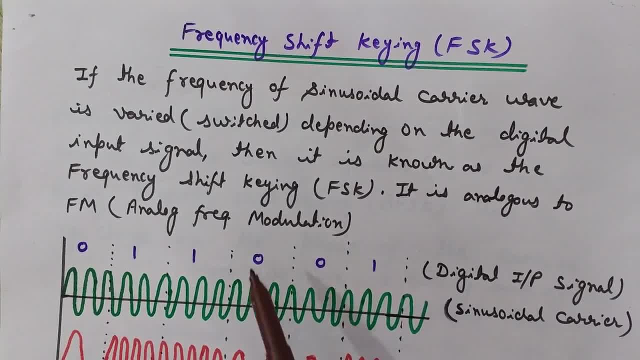 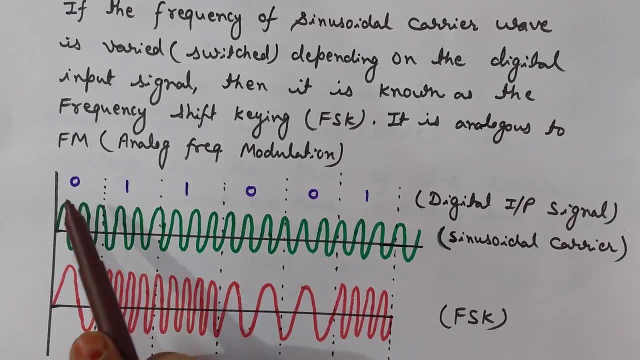 as binary FSK, Because here we vary the frequency of this carrier wave according to the variations in the input signal, digital input signal. As you can see here that this sinusoidal carrier wave has constant amplitude and constant frequency. Its frequency is not varying And its amplitude is. 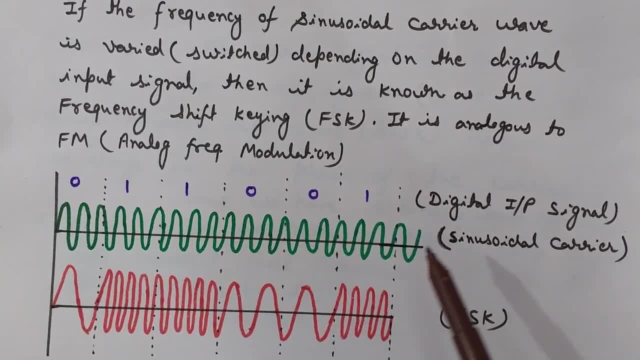 constant. But after modulation, when we do FSK, we just vary the, we just switch the frequency of this carrier wave as per the digital input signal, this digital input stream of zeros and ones, Since we have only two symbols, zero and one. So we will discuss here the binary phase shift keying. It is 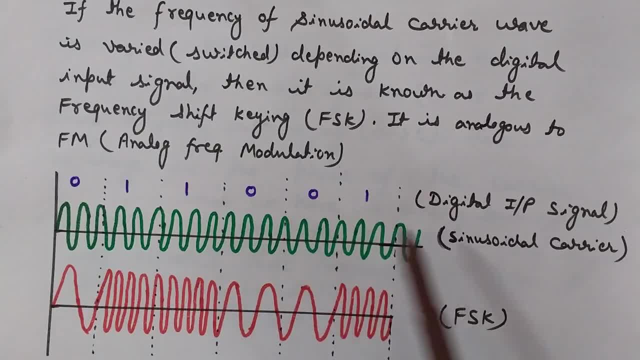 known as BFSK. As you can see that in frequency modulation also, if we talk about the continuous wave modulation, its examples are FM, AM, PM, etc. So this FSK is analogous to FM, Because in frequency modulation we just vary the frequency of the carrier wave according to the modulating. 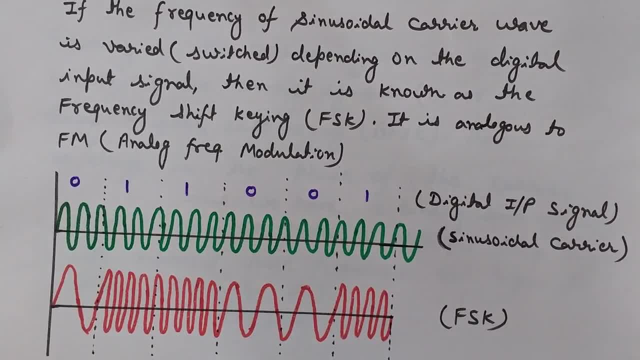 signal. But the difference is that in continuous wave modulation, FM, the modulating signal is in analog form. But in digital form of this, that is, FSK, the modulating signal is digital input, Okay, And the carrier wave is analog in both of these cases. in continuous wave modulation, 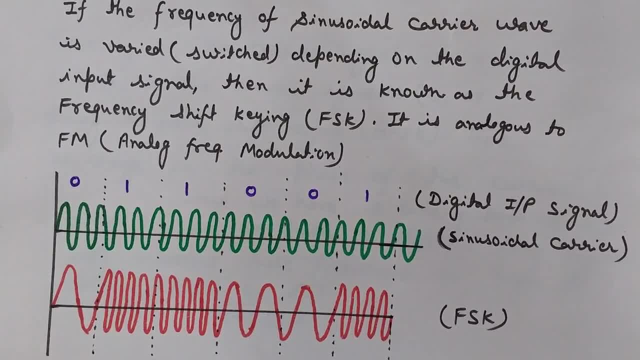 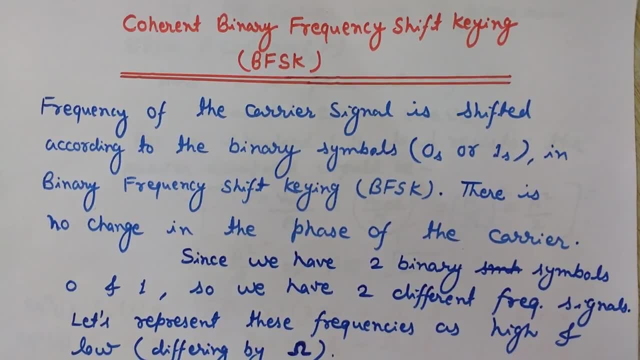 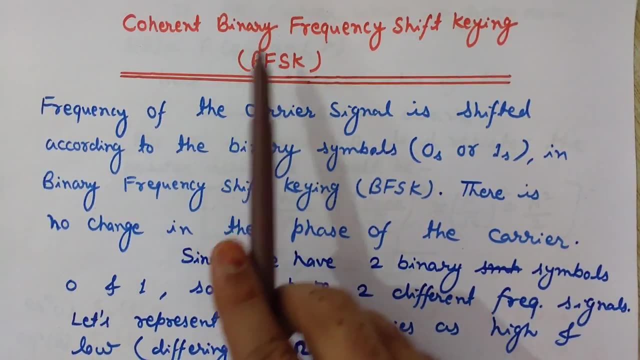 and in digital modulation. Okay, So now we understand the basics of FSK. So now it's time to understand the coherent binary frequency shift keying BFSK. As I told you, that binary means two: Here we are using zero and one at the input end, at the 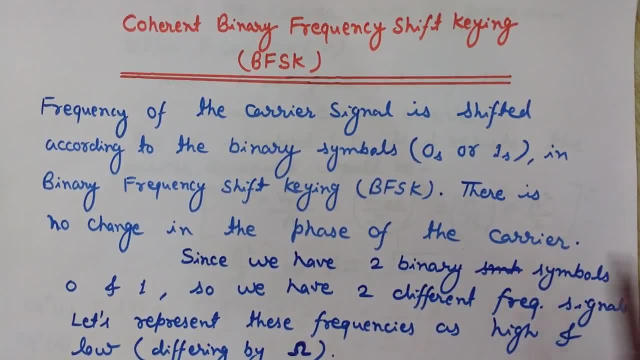 as the modulating signal, So it is called as binary And in binary frequency shift keying, since we vary the frequency of the carrier wave according to the binary symbols, since there are only two types of binary symbols here, zero and one, So we get two types of 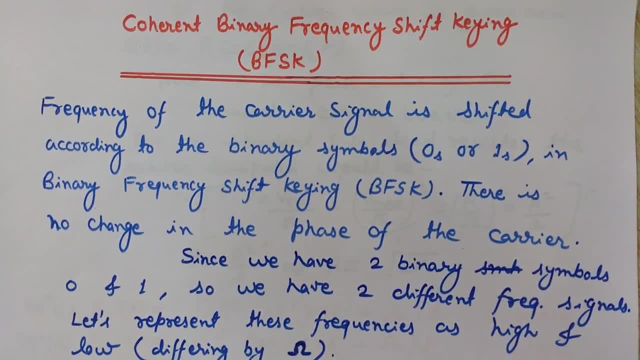 frequencies in the wave form of BFSK: The frequency component that is corresponding to the zero- we're having a lower frequency- And another component corresponding to the corresponding to digital input. one will have correspondingly higher frequency component. So the wave form has two different frequency signals. If we represent these frequencies, 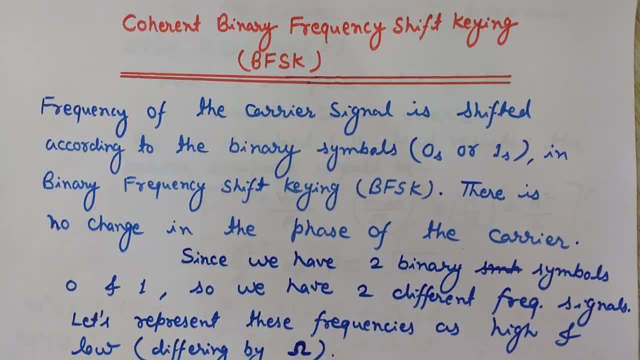 as high and low and we, for mathematical purpose, we are using omega to distinguish the difference in high and low frequencies. If the frequency of this carrier wave is 2piFC, then 2piFC plus omega will correspond to the high frequency component, while 2piFC minus. 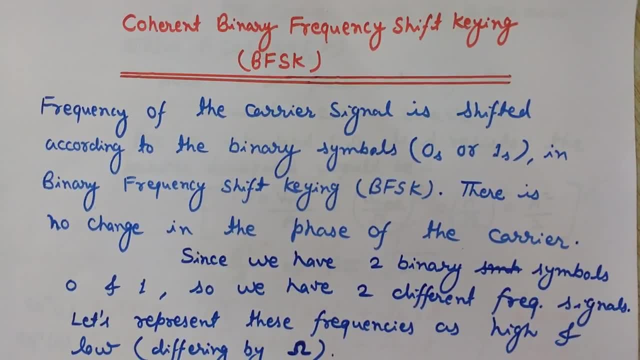 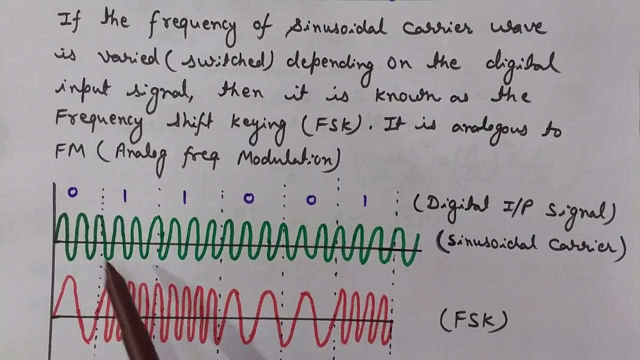 omega will correspond to the low frequency component. So let's understand and let me explain to you the mathematical expression and the derivation of FSK, BFSK. Okay, You can understand this concept of FSK from this wave form also, because here it is zero And we have- we can see that here- the frequency. 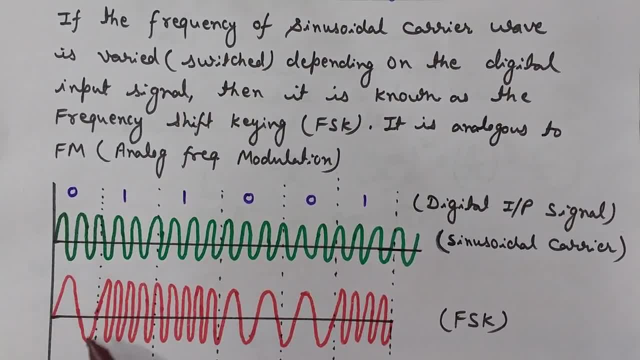 Frequency is low. Okay, What is frequency? Frequency is the: how many cycles, how many cycles or wavelengths are passed per second. So you can see here that here it is one and one. These two inputs are one and one in digital inputs. So here the frequency is high. It is, it has high frequency, Okay, More number of cycles are passing per second. But again, when it comes to zero, it switches to zero. Then we have 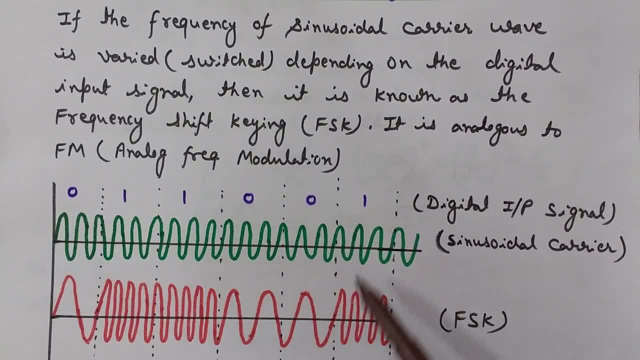 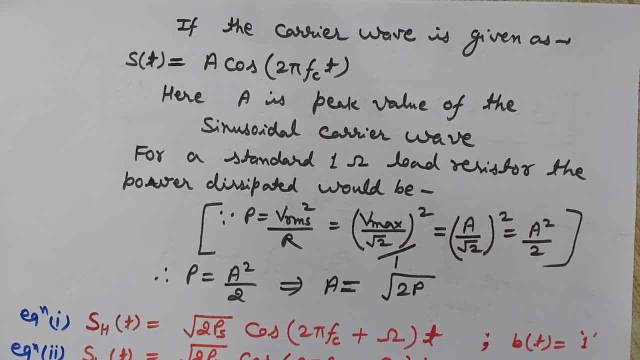 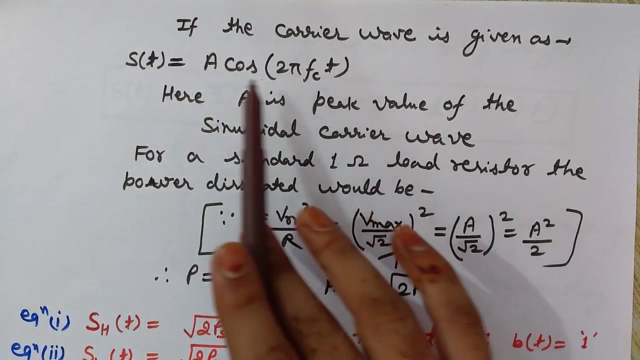 low frequency from here to here, where we have zero, And again for one we have high frequency component. So it has been modulated. The carrier frequency has been modulated according to the digital inputs, So it is FSK frequency shift king. Okay, Now again come to the mathematical expression. So let's suppose that the carrier wave is given by ST equals to a cost of two pi FCT. here is the peak value, maximum amplitude of the sinusoidal carrier wave, And this is 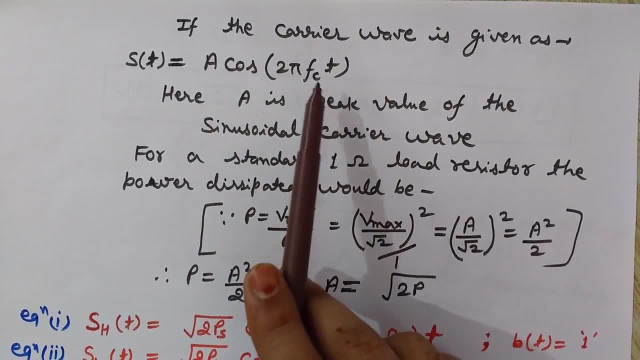 cost means sinusoidal wave and two pi FC. What is FC? It is the frequency of the carrier wave, T is time. So for if we consider a standard one ohm load resistor, then the power dissipated would be. we know that power is VRMS squared divided by R. Okay, And VRMS is what it is: V max by root two. Okay, Since we know that V max is VRMS into root two. So it is VRMS. is V max by root two, whole square. So 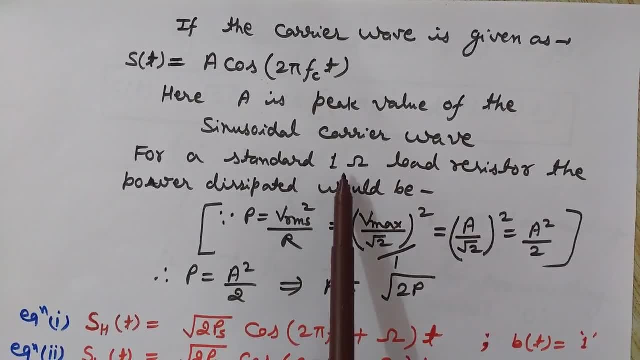 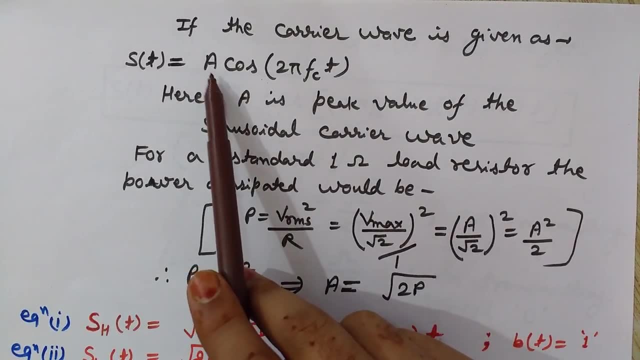 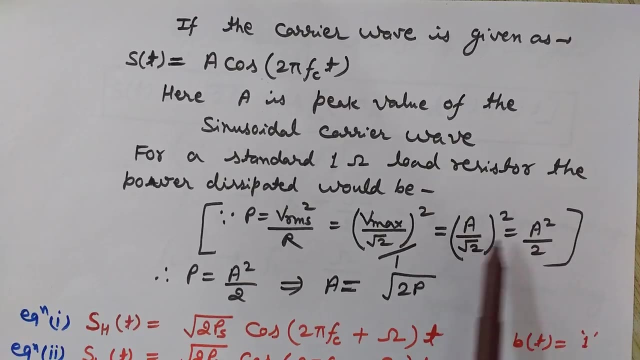 same. this divided by R, R is R is here. We are taking one ohm, So it is one ohm And we know that V max is what V max. from this equation We know here we get the maximum amplitude, So V max is a. So replace this V max by a and root two and whole square. This is divided by one means. it is simplified to a by root two, whole square. If you solve this, you get a square by two. So we get power is equals to a square by two. 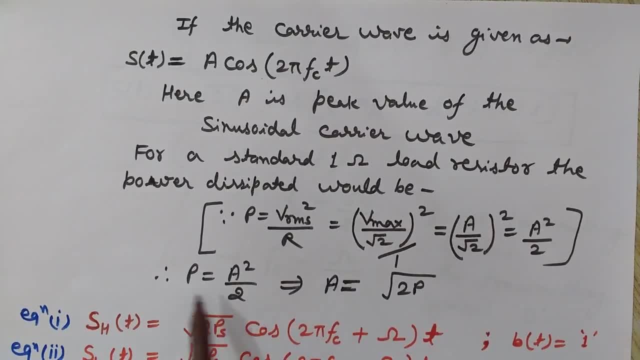 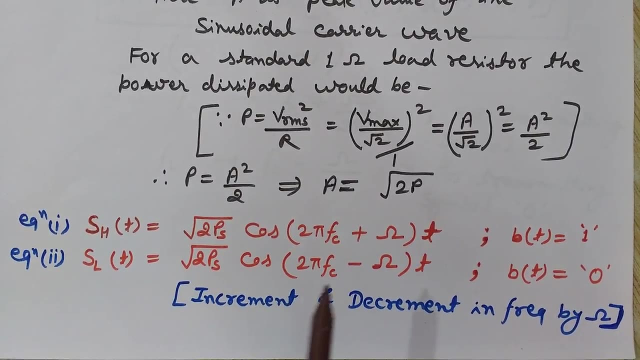 Okay, And from this we have a is equals to under root of two P. So in this equation just replace this a amplitude, maximum amplitude by root two P. P is the dissipated power here. So as we have already seen that in FSK in binary phase shift keying we have only two frequency components because we have only two binary symbols according to which we vary the carrier frequency. So just replace. just see that here at the place of 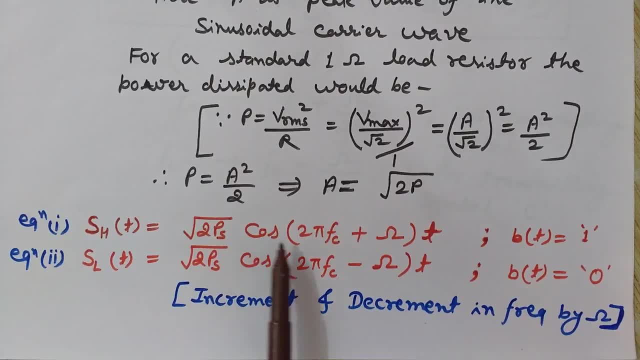 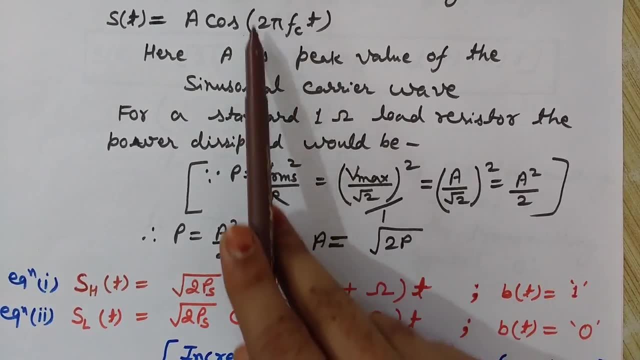 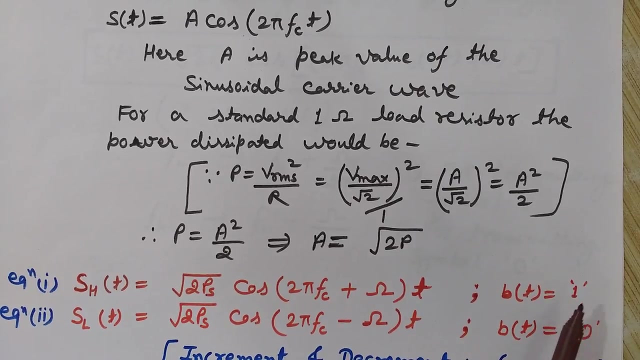 a. We have under root two P S Cause of two pi FC. This FC, since frequency of the carrier wave is two pi FC, We know that two pi FC is the omega. Omega is two pi FC. So it is two pi FC plus omega. If we are taking the high frequency component, which is corresponding to binary symbol one, Okay, And for binary symbol zero, this is the lower frequency component- Decrease the frequency of the carrier wave. 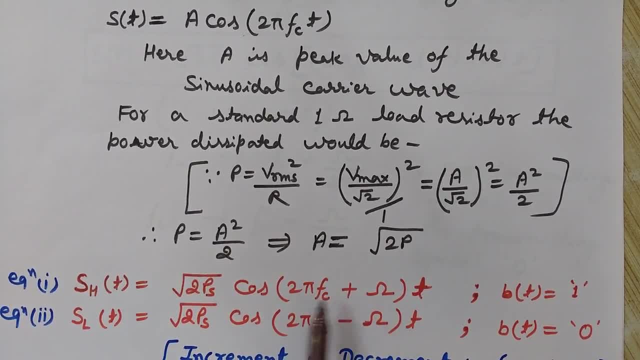 That is two pi FC by omega. So it is plus omega for high frequency component, corresponding to one. Okay, Binary input, one and zero, corresponding to zero binary input. We have minus omega, two pi FC minus omega And this is nothing but T, Okay. So just we get two frequency components, Okay, Two pi FC plus omega and two pi FC minus omega, corresponding to zero, corresponding to one and zero respectively in BFSK. Okay, 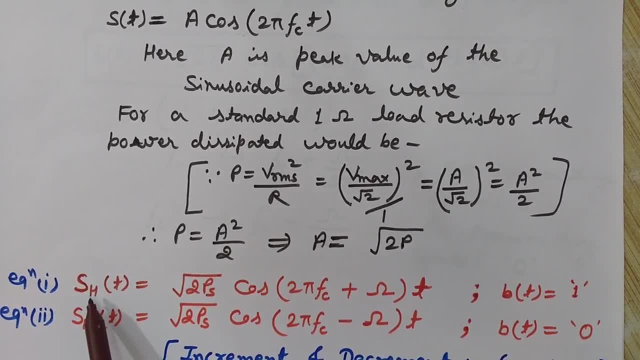 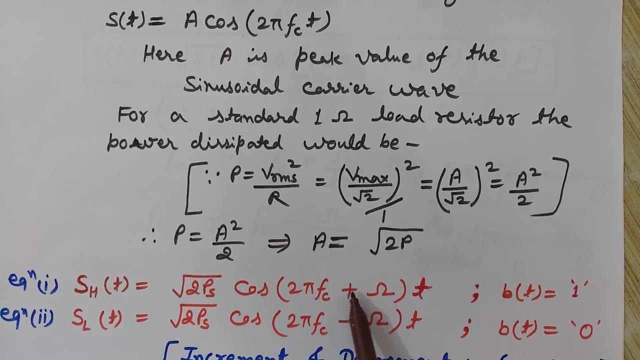 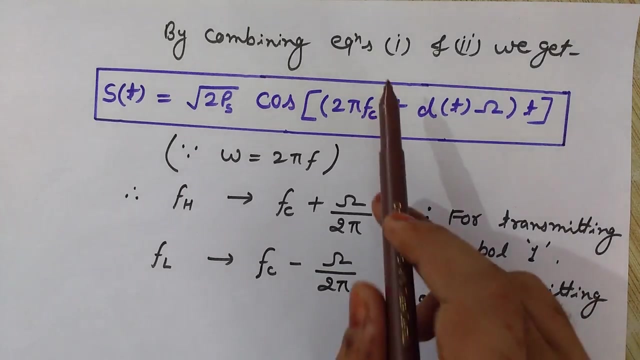 So this is H, SH represents the higher frequency component, and this is SL, equation one and equation two. Now if we combine these both of these equations, equation one and two, then we want to write a single equation where we can incorporate this plus and minus in one equation. So let's do this. So by combining these equations one and two, we get under root two P S Cause, two pi FC plus DT omega. 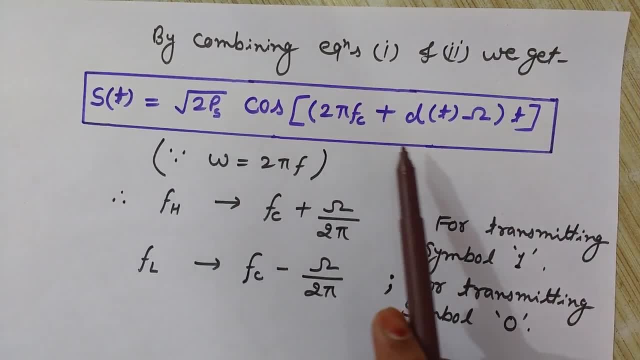 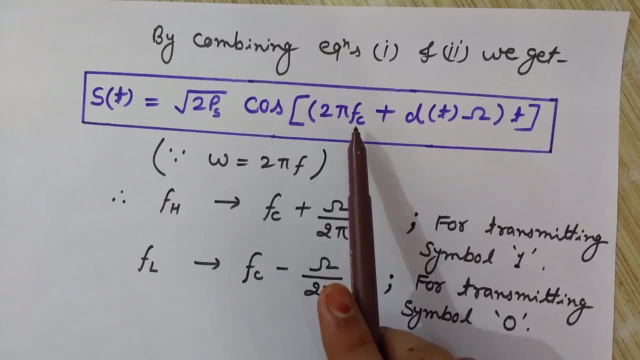 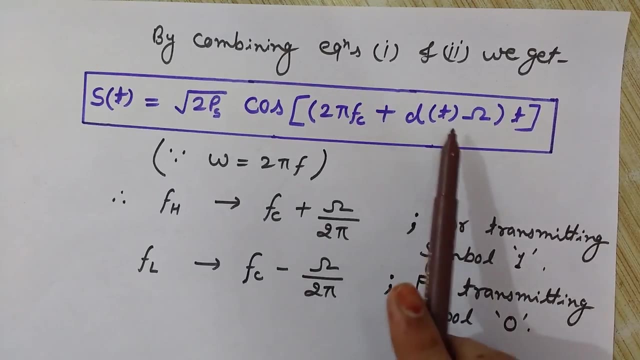 And T. We have done nothing special here, Just we have combined these two equation. in the first equation It was two pi FC plus omega and two pi FC minus omega for the second one. So we have replaced this DT plus and minus with DT. Okay, This will take care of this. plus minus, Okay, Plus and minus. So we understand that omega is two pi F. Okay, And F is nothing but omega divided by two pi. So 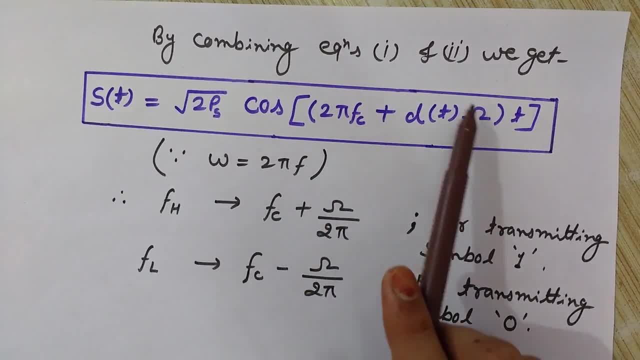 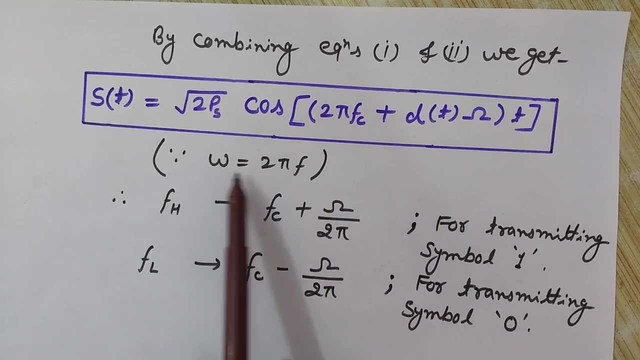 if this is the omega two pi, FC is omega and here it is omega part, omega and omega. So if I want to write the frequency component, then F. we know that it is omega divided by two pi. So just to get the high frequency component, we have FC: the frequency of the carrier wave plus the frequency incremented by omega by two pi. Since F is what F is, omega divided by two pi, So C plus omega by two pi. This is a frequency component for transmitting omega.